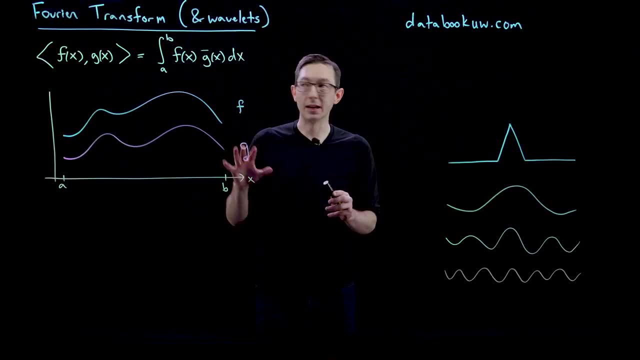 of x times complex conjugate of g of x. but for real value data, for real valued functions- f and g- the complex conjugate of g is just g, so you can kind of forget that. so don't worry about that right now. 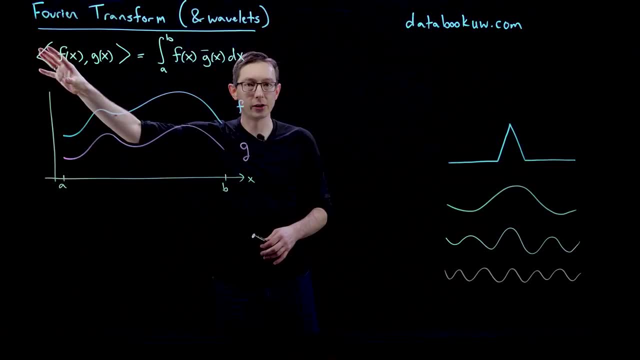 Ok, so this is how we define the inner product of two functions. This essentially tells me how similar these two functions are, just like the inner product of vectors tells me. you know, if my two vectors are orthogonal, then my inner product is zero. 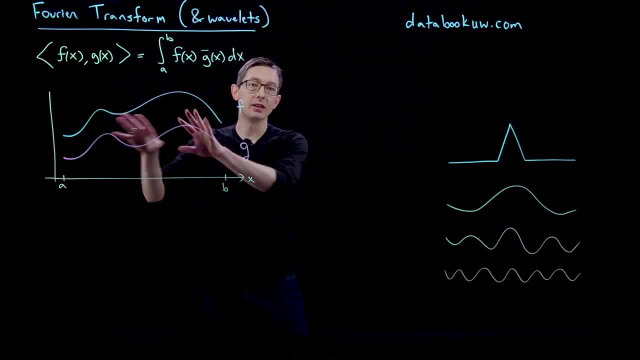 If they're very well aligned, I have a large inner product. It's exactly the same thing with these functions, So the two that I drew here are actually very close to each other, so they should have a large inner product when I multiply them and integrate from a to b. 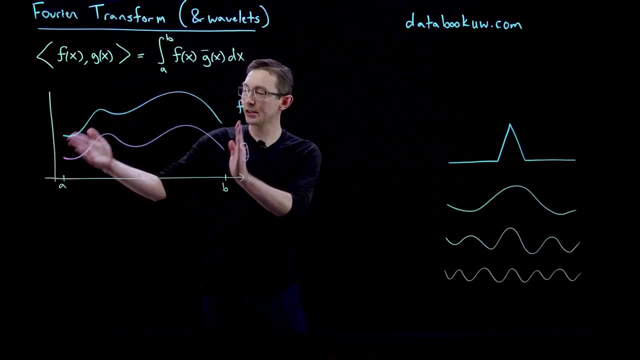 Ok, but what I want to show you now is that if we discretize these functions at a discrete set of x locations and we collect data vectors of the function evaluated at those positions, then this inner product essentially comes from that inner product of sampling. so I'm going to do that right now. 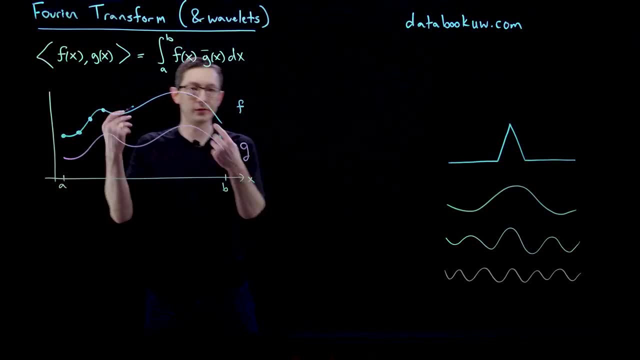 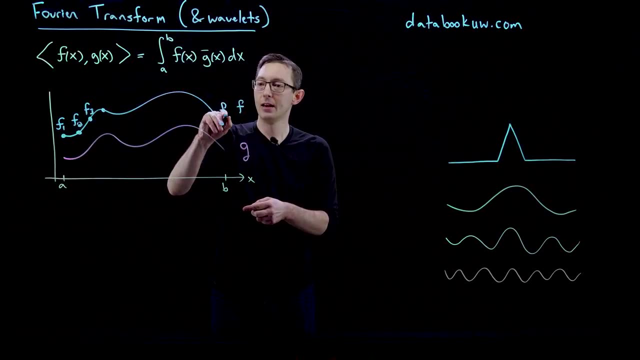 So what we're going to do is we're going to sample this function f at a bunch of discrete locations: f1,, f2, f3, and so on and so forth, all the way up to fn. so I'm I'm gonna have n samples of this function. 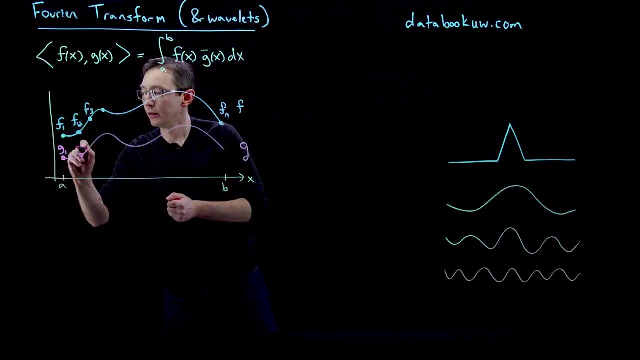 I'm gonna do the same thing with g, so g one, g two, g three, and so on and so forth, all the way up to gn, And I'm going to be sampling these at regular intervals: x one, x two, x three, dot, dot, dot. 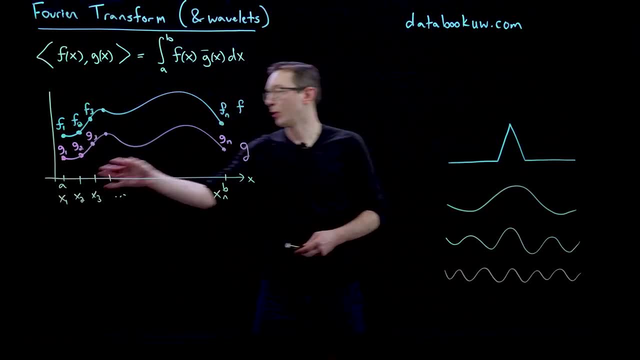 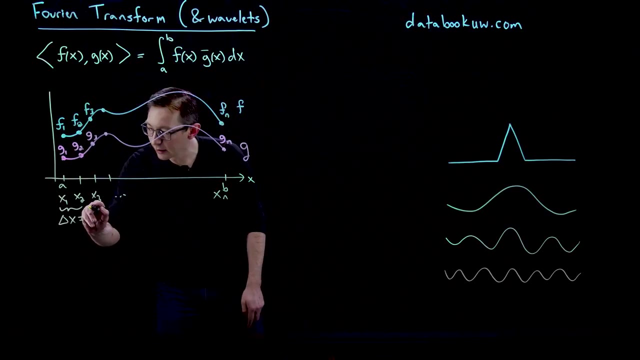 all the way up to xn. okay, And so I'm going to, for now, just assume that there's a constant delta x that I'm using to sample between these points. okay, So I think I would have something like: delta x is equal to b minus a divided by n minus one. 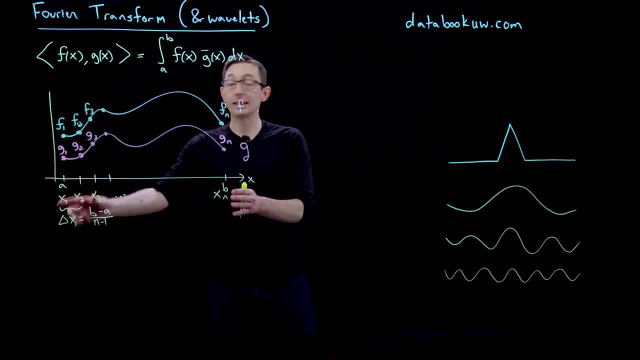 something like that. okay, So as I increase n or as I decrease delta x, I increase the number of sample points n that I have. okay, And so what we're gonna do is we're gonna think about the inner product of data vectors. 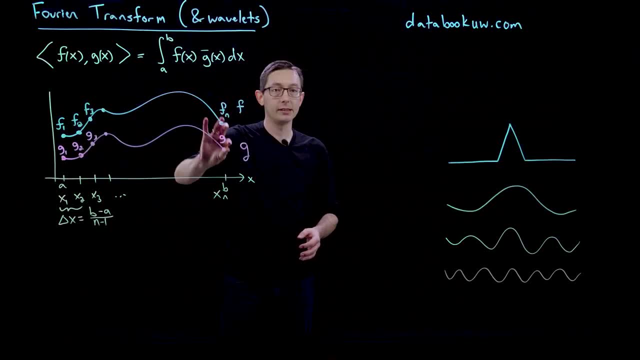 containing these sampled points f and these sampled points g, and I'm gonna show you that, as you take the limit, as delta x goes to zero, as this becomes infinitely finely resolved, as you recover these functions, then you recover this function definition. 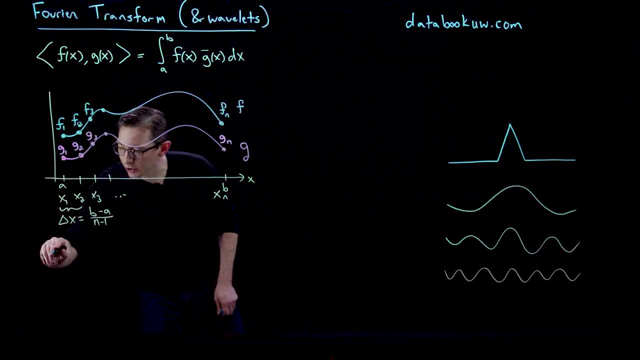 of an inner product. okay, So let's do that. So my f function is: I'm just gonna put an underbar to denote that this is kind of a vector of data, like we're used to seeing an n-dimensional vector containing f, one, f two, dot, dot, dot, dot. 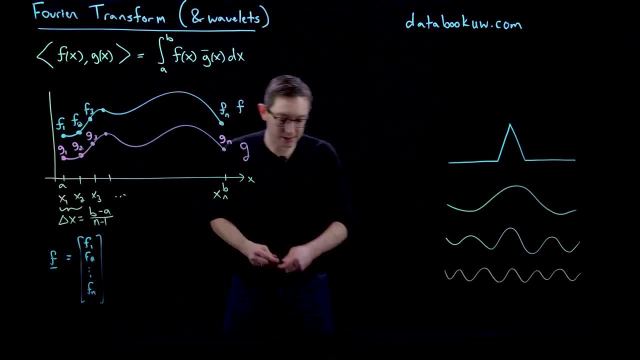 dot all the way down to f, n, And similarly I'm going to have g. underbar is g one, g two, dot, dot, dot all the way down to g n. Good, Now, it's relatively straightforward to take the inner product of these vectors. 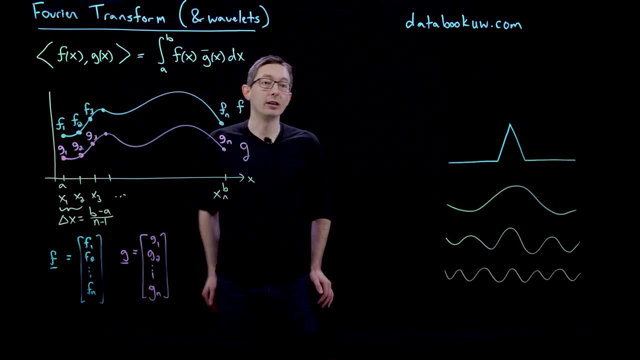 We know exactly how to do that. We have lots of intuition for how to compute the inner product of these two vectors, And what I'm gonna show you is that when you do that and then you take n goes to infinity, or delta x goes to zero, you recover this exactly okay. 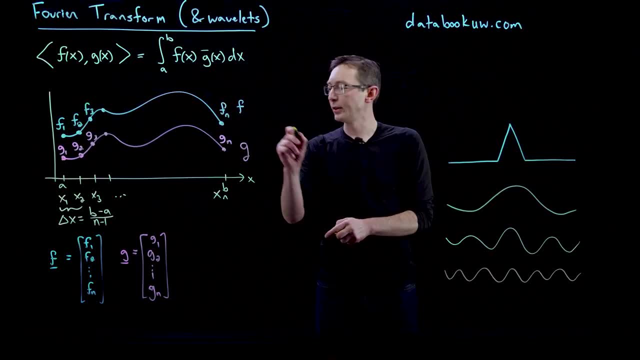 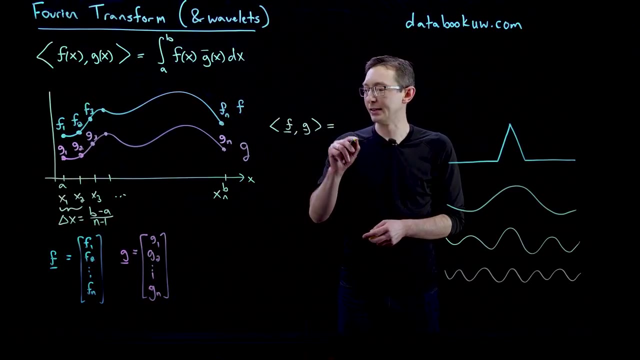 So let's do that right now. So what we're gonna do is we're going to take the inner product of vector f with vector g, kind of my data vectors here, And we know that this is going to be. I'm gonna just define this as g transpose f. 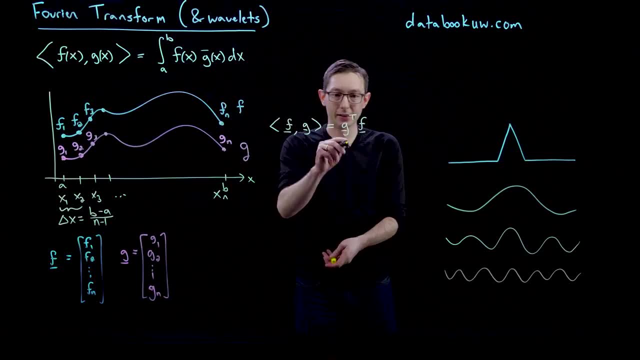 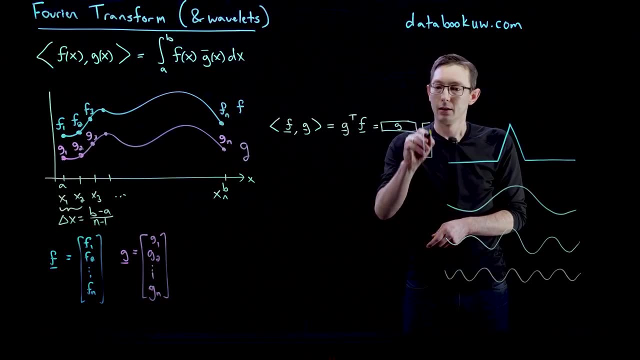 So what that essentially means is: I take g, I knock it over on its side. so let me draw a picture. It looks like g as a row vector times f as a column vector. okay, And what that means is that I take the first element. 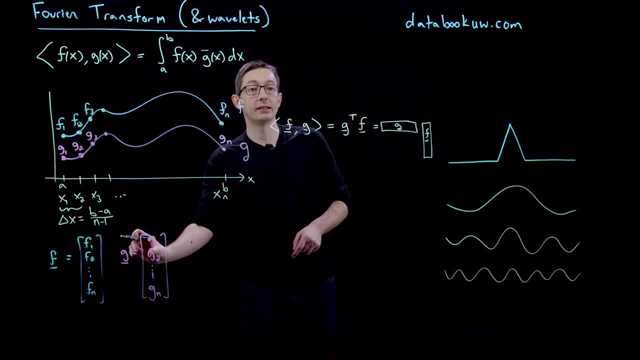 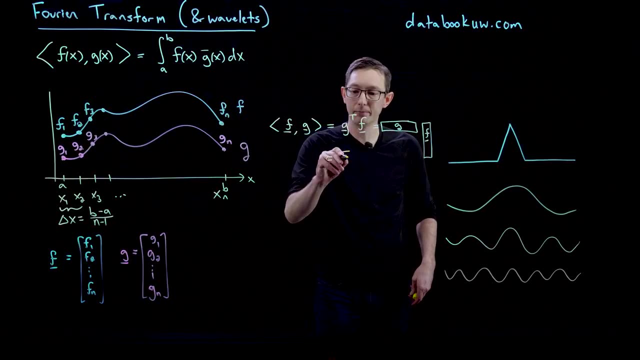 of f one times the first element of g, one plus the second element of f two plus the second element, g two plus f three, g three plus f four, g four and so on and so forth. okay, So this is a sum from k equals one to n of f one. 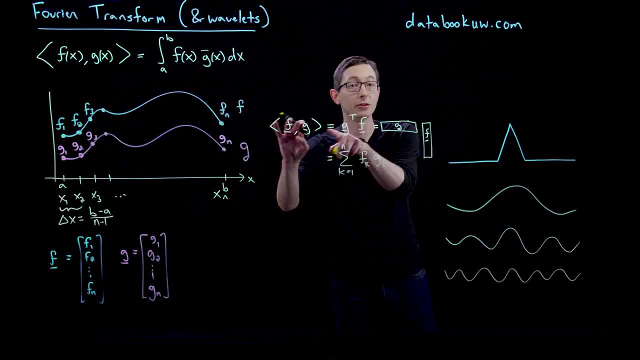 plus f, k, g, k. And again, if this was complex value data, this would be g bar and this would be complex conjugate transpose. I'm just gonna neglect that for now, but I want you to remember that if this was complex data, 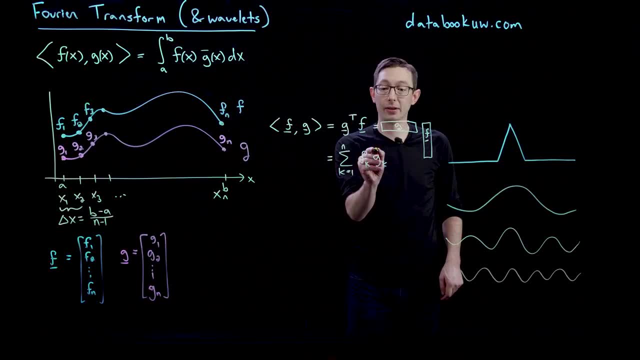 this would be complex conjugate transpose and this would be a complex conjugate on all of these little g's. okay, Now there's a little bit of an issue here, as far as I see it, which is if I double the number of data points, 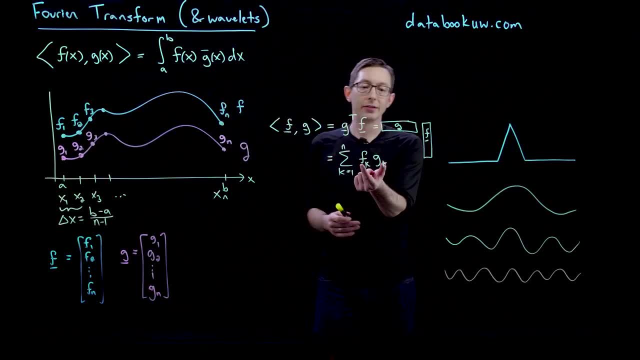 if I have two n's, if I have two n's, if I have two n's, if I have two n data points instead of just n, this gets twice as large because I'm adding up twice as many things. So that's a little strange. 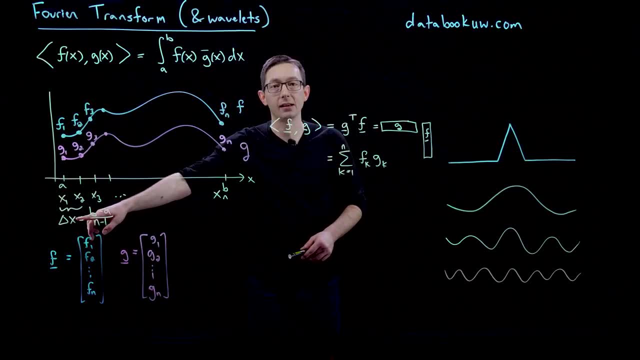 So what we're going to do instead is we're going to normalize this by delta x, which is going to make it so that, if I double the resolution, this number doesn't get twice as big just because I have twice as many data points. okay, 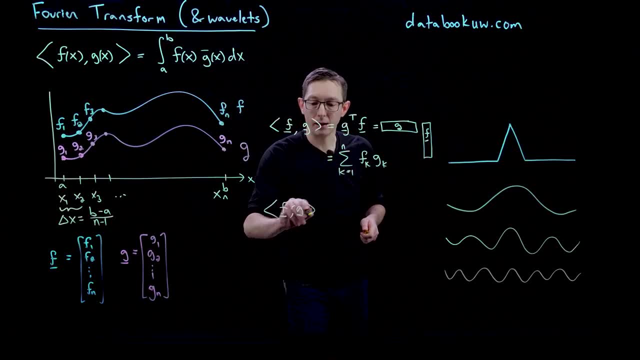 So if I look at my f- g on my data vectors times delta x, now what I have is this: equals my sum from k, equals one to n of f of k, g, k times delta x. Now what I'm going to say here is that f- k 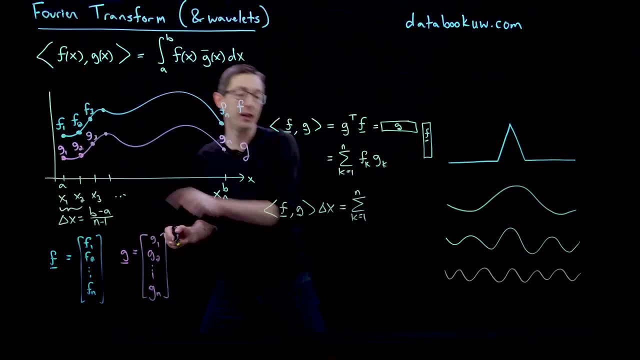 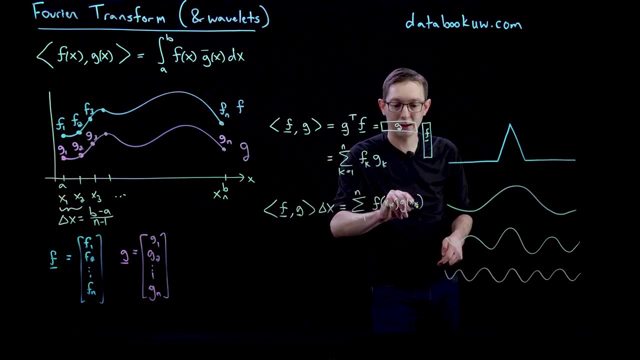 we know that f- k is just f evaluated at x k. So I'm going to say that this is f at x k, g at x k times delta x, And so this is where kind of it all comes together. If I this is just the Riemann approximation. 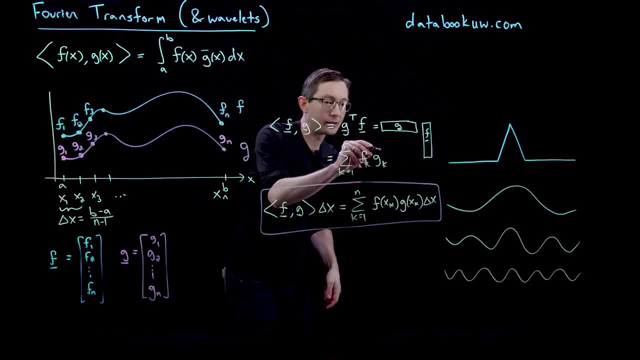 of my continuous integral up here. Remember, if this was complex value data, these would have bars, bars. this would be a complex conjugate transpose. And so if I take the limit as delta x goes to zero, so I have infinitely fine resolution. 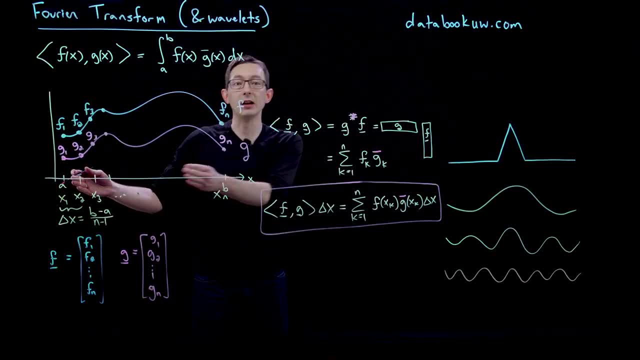 this vector becomes infinitely tall and it contains the whole function from a to b. then this Riemann approximation becomes my continuous integral formula. So I just wanted to show you that this definition of the inner product for functions- again it tells you exactly the same information. 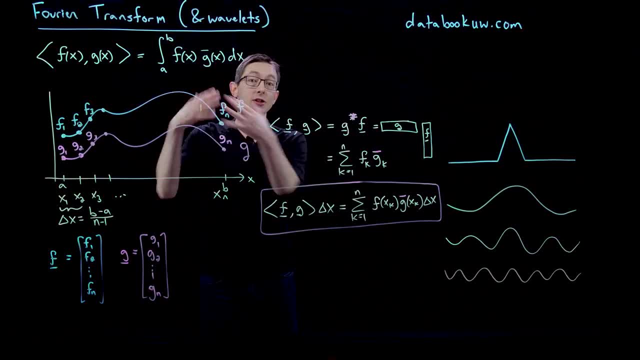 that the inner product of vectors tells you. It tells you how close these two functions, f and g, are to each other, how aligned are they in function space. But there's nothing kind of magical happening here. This is just what you would get if you took the inner product of vectors of data.